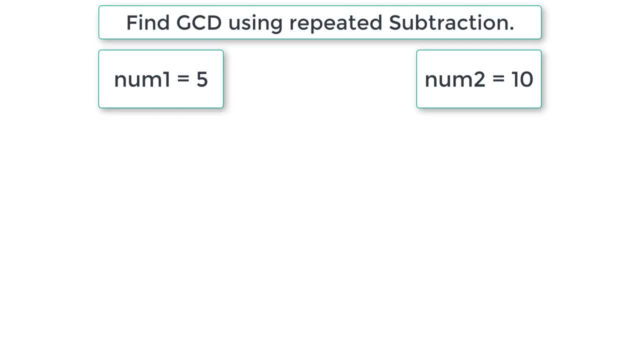 not equal yet. So num2 is greater. So num2 minus num1 will be stored inside num2.. Now num1 and num2 are equal. So greatest common divisor of 20 and 15 is 5.. Simple. Let's write the C program for this. 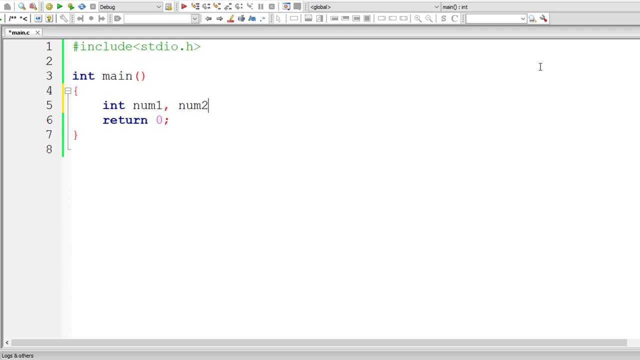 I'll take two integer variables: num1 and num2.. I'll ask the user to enter two positive integer numbers. One drawback with this is, since we are using subtraction here, we can't calculate GCD for negative numbers. Okay, So enter two positive. 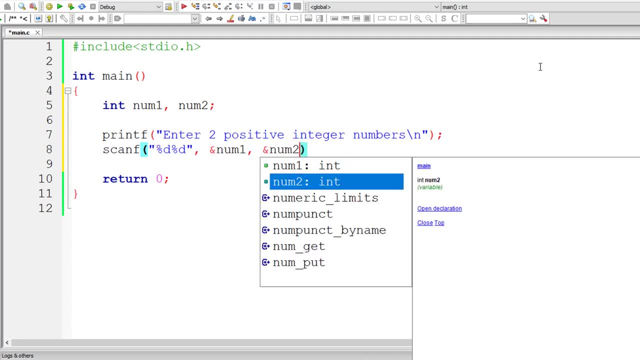 integer numbers And we will store that inside address of variables, that is, integer variables num1 and num2.. I'll print a statement here that is half of the result here, Just a statement, Because we will be modifying the values of num1 and num2.. At the end we won't get these numbers, So let me print it. 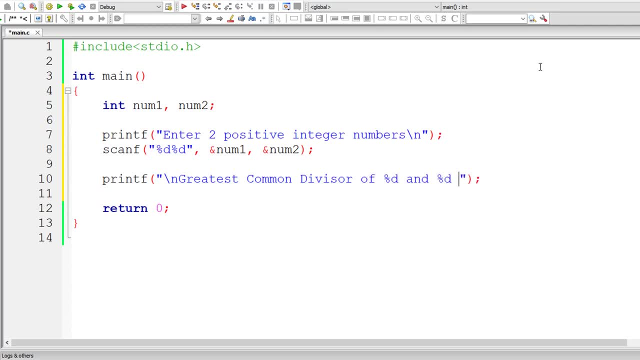 now itself. So the greatest common divisor of %d and %d is, with a space with no newline character at the end of num1 and num2. at the end you will know why i did this. so, while num1 is not equal to num2, 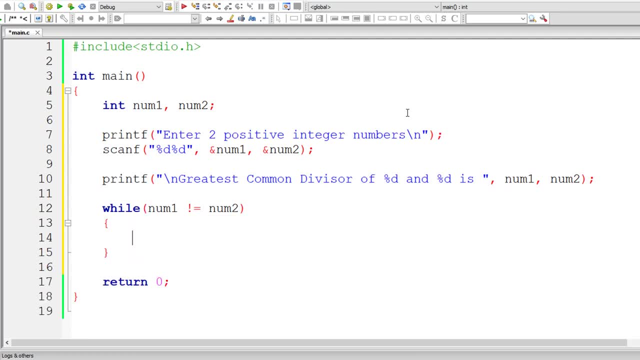 this is the condition. so until this is true, keep on executing this, iterating this while loop. okay, until num1 is not equal to num2, keep iterating through this while loop. so if num1 is greater than num2, if this condition is true, get inside. if block, then num1 is equal to num1. 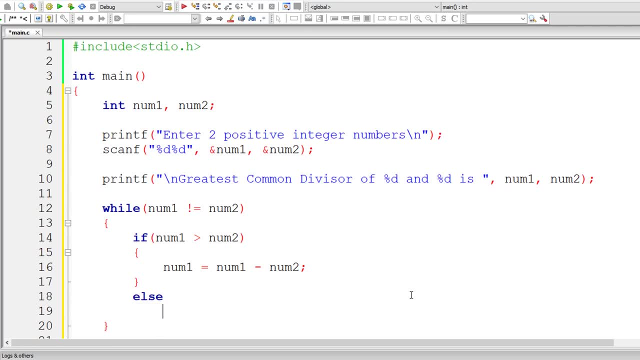 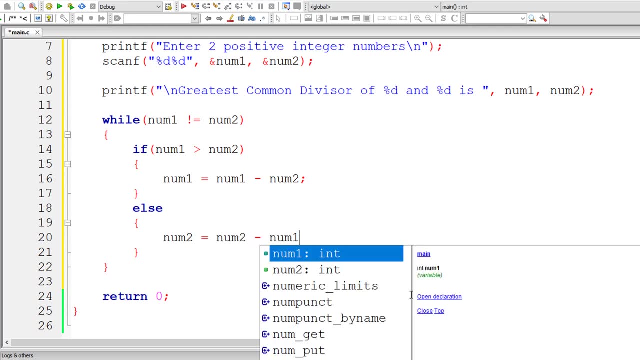 minus num2, simple, else. else num2 is big, right, so num2 is equal to num2 minus num1. simple thing. once num1 and num2 are equal, the condition is false and while the control exits this while loop. so i will continue writing this printf statement here and print the result with: 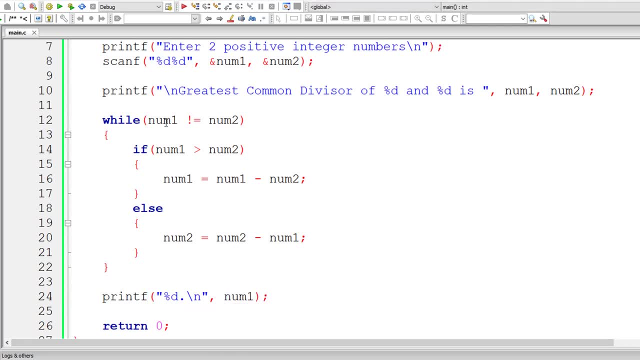 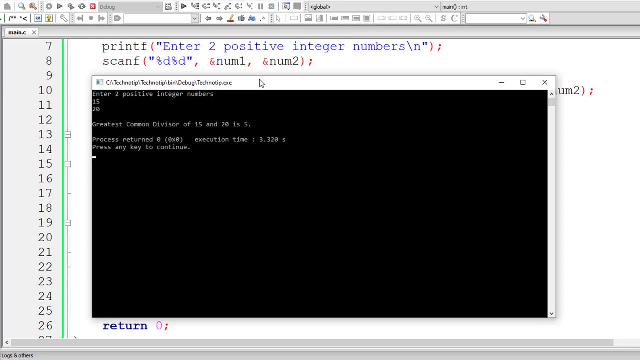 a new line character, so result will be present inside either num1 or num2, because this is the condition. so i will continue writing this printf statement here and print the result. this while loop exits only when both num1 and num2 are equal. so let's check the result. 15 and 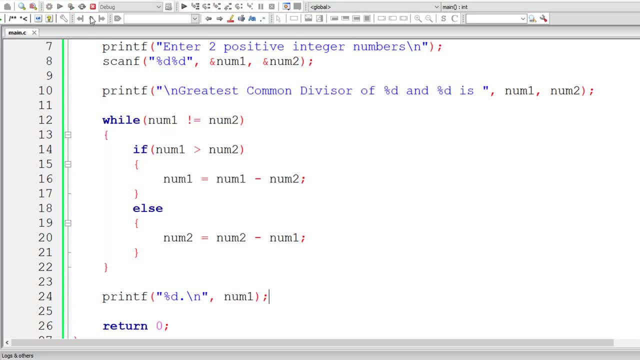 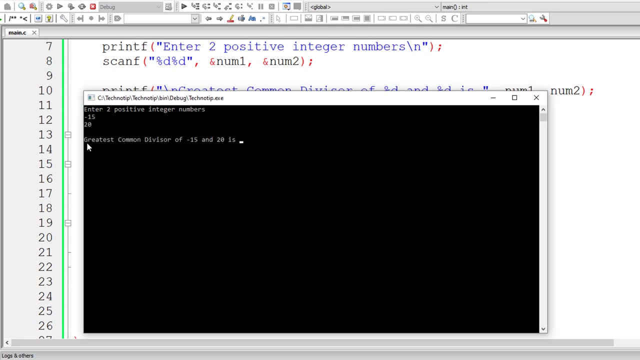 20 should give 5 as the greatest common divisor. let me reverse the input, that is 20 and 15. it should give 5 as gcd as well and it's working for negative numbers. it doesn't work minus 15 and 20. let's try that greatest common divisor of minus 20 and minus 15 and 20 is. it doesn't print the. 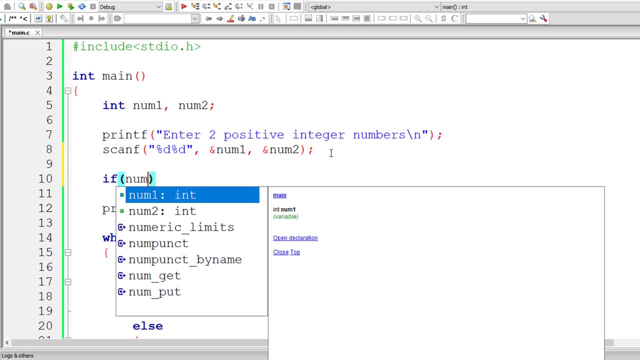 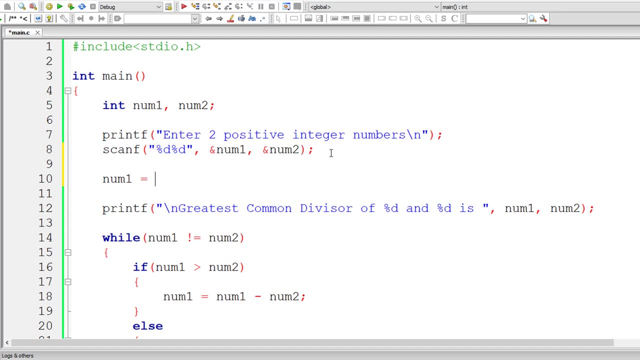 result. so to solve this problem, let's try this problem. let's try this problem. let's try this problem. solve that. let me write a if block and convert the negative number to positive, or else i'll write. i'll simply write a ternary operator. the condition is if num1 is less than zero. okay, 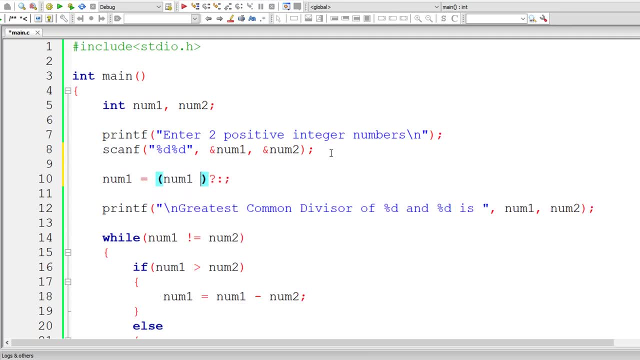 what does that mean if num1 is less than zero? what does that mean? that means the number num1 entered by the user is is a negative number. in that case, return minus num1, that's it simple. or else simply return the num1. so what's the logic behind this minus num1? 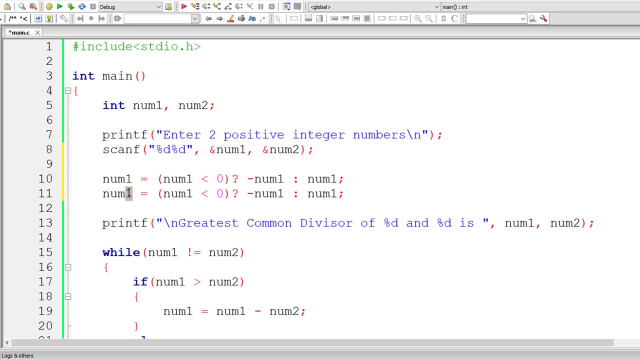 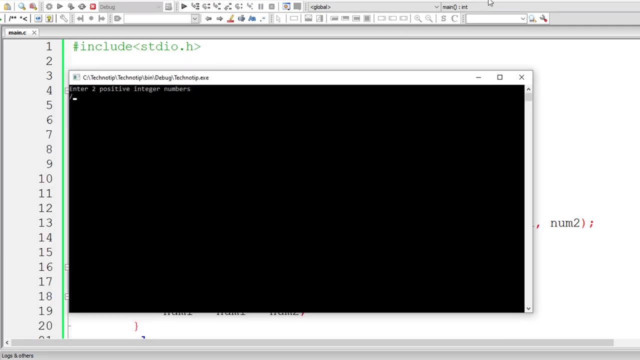 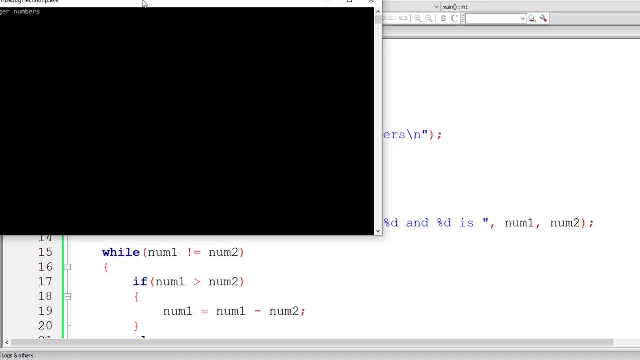 if the user has entered minus 15. so minus of minus 15 is plus 15, simple logic. let's do the same for num2. so at the end we will have num1 and num2 as both as positive value, irrespective of what sign user enters. so minus 15 and 20 should give 5 as gcd, and the same works for 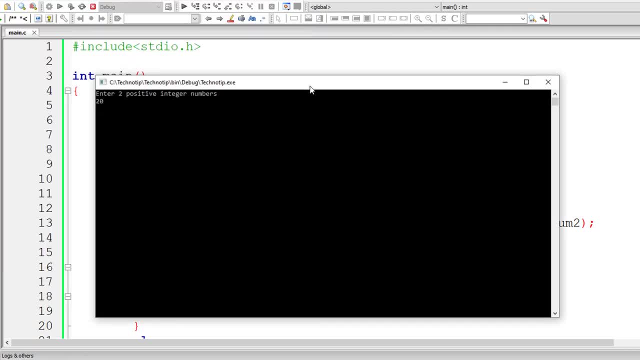 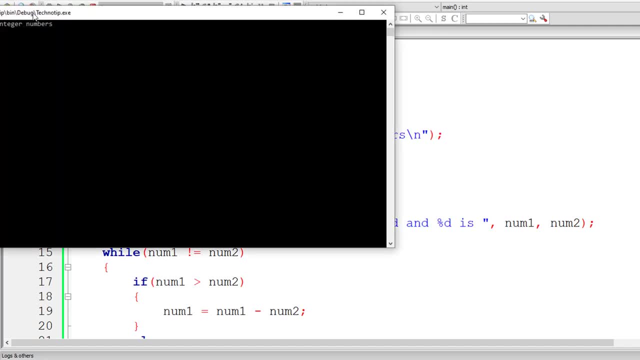 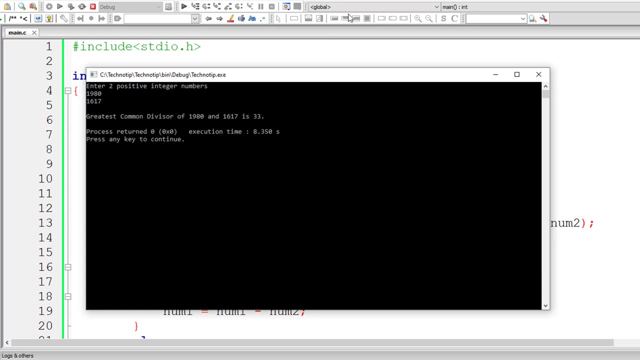 20 and minus 15. let me give minus 15. it's still gives 5 as reddish common divisor. so let me try for one more input. i'll give first value as 1980 and second value as 1617. so 33 should be the gcd. and it's working. that's great. this is how we find. 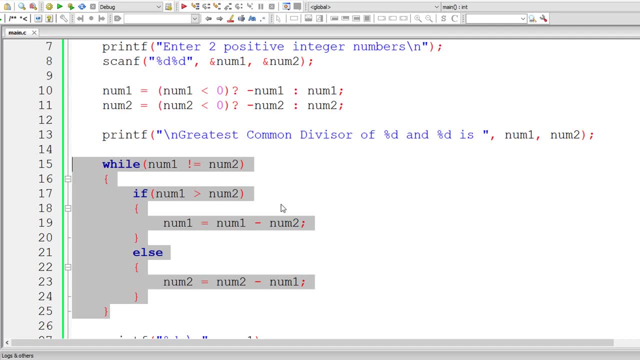 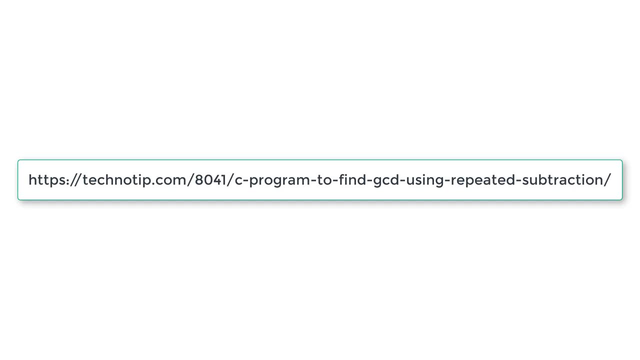 gcd of two numbers using repeated subtraction method. so this is the logic. please visit the link present in the description section of this youtube video for source code notes and discussion about this topic, and i'll see you in the next video. bye, bye. stay subscribed to our youtube channel and blog, and please share this video with your friends on. 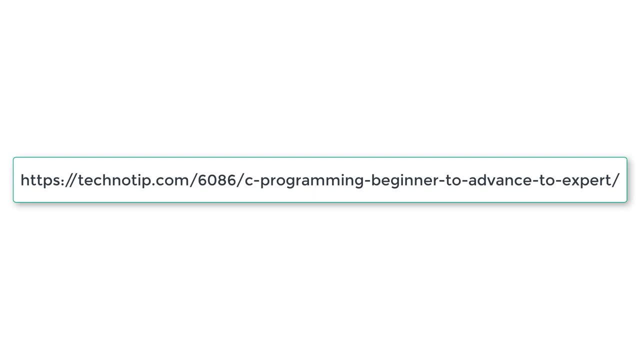 your whatsapp, telegram, wechat or maybe twitter, linkedin facebook, etc. and please do not forget to like this video on youtube. thank you.